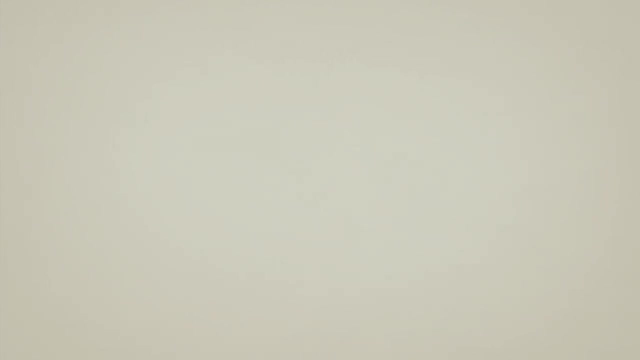 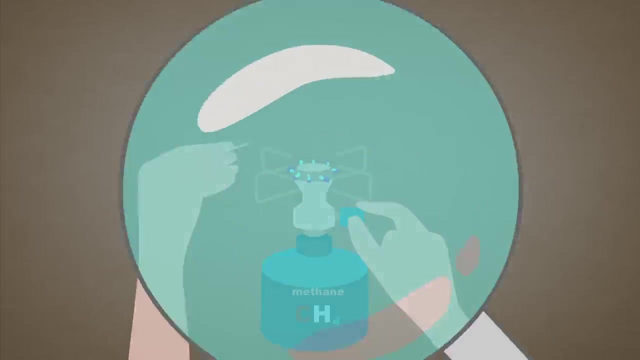 This here is methane, most commonly associated with cow flatulence, but also used for rocket fuel. If we add some oxygen and a little bit of energy, like you might get from a lit match, it combusts into carbon dioxide, Carbon dioxide, water and even more energy. 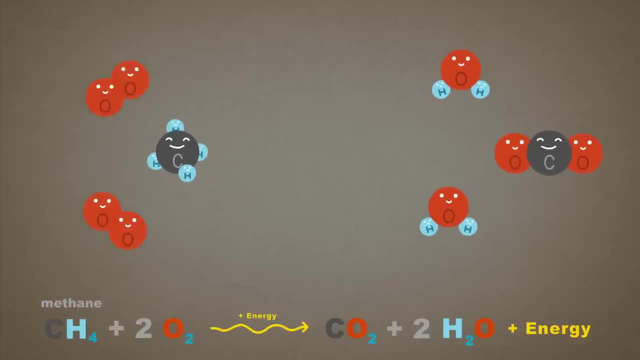 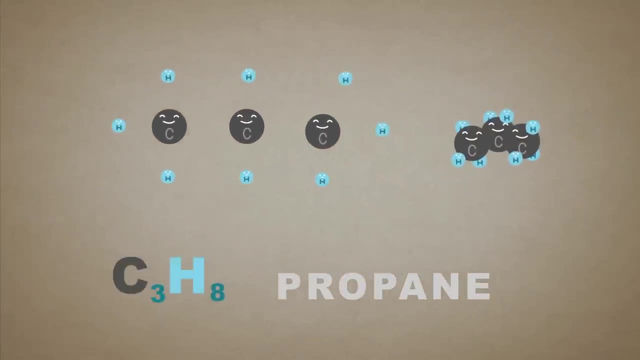 Notice: our methane started with 4 hydrogen and at the end we still have 4 hydrogen captured in 2 water molecules. For a grand finale, here's propane, another combustible gas. We add oxygen, light it up. 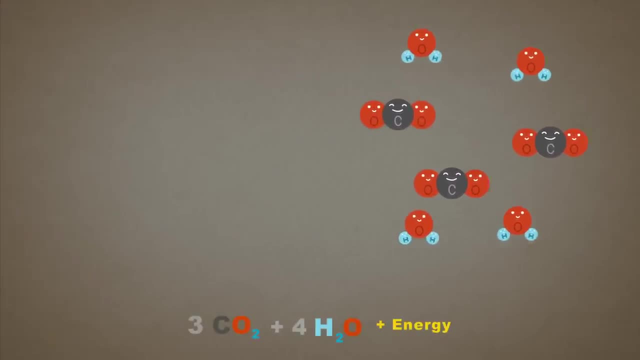 and boom, more water and carbon dioxide. This time we get 3 CO2s because the propane molecule started with 3 carbon atoms and they have nowhere else to go. There are many other reactions we can model with this small set of atoms. 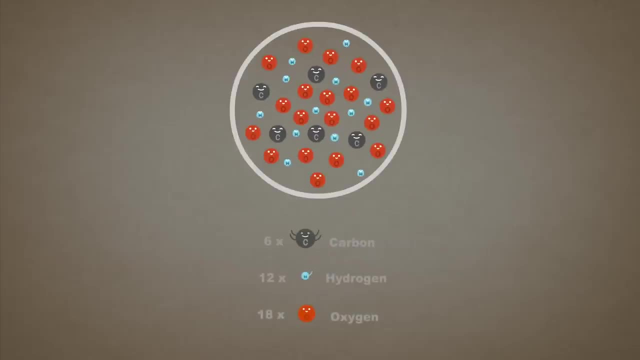 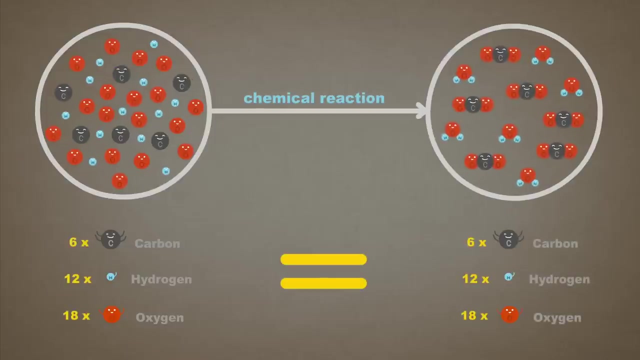 and the law of conservation of mass always holds true. Whatever matter and energy go into a chemical reaction are present and accounted for when it's complete. So if mass can't be created or destroyed, where did these atoms come from in the first place? 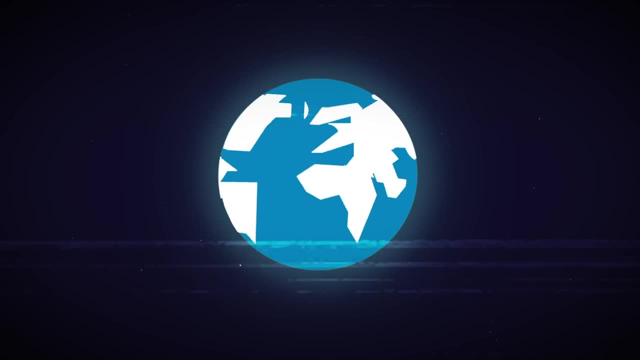 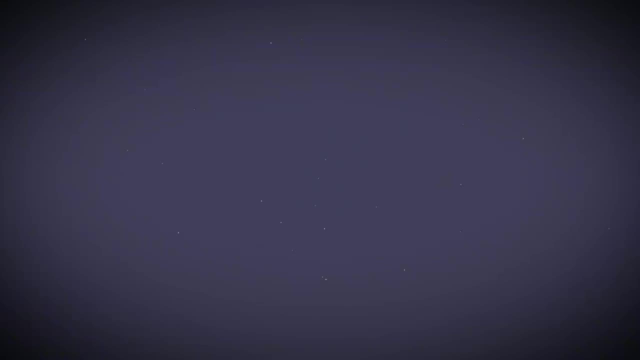 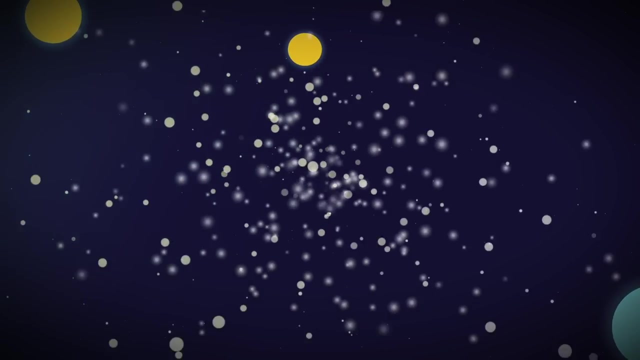 Let's turn back the clock and see Further, further, further, Too far. Okay, there it is The Big Bang. Our hydrogen formed from a high-energy soup of particles in the 3 minutes that followed the birth of our universe. 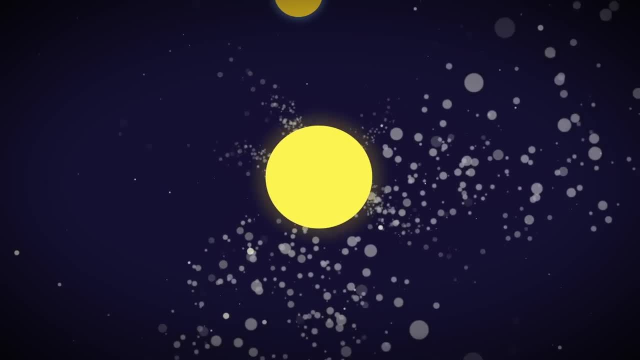 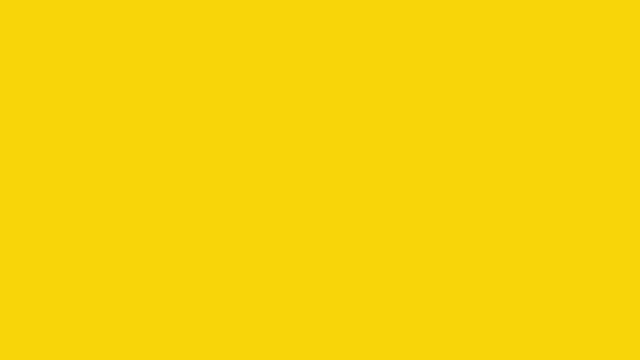 Eventually, clusters of atoms accumulated and formed stars. Within these stars, nuclear reactions fused light elements such as hydrogen and helium to form heavier elements such as carbon and oxygen. At first glance, these reactions may look like they're breaking the law. 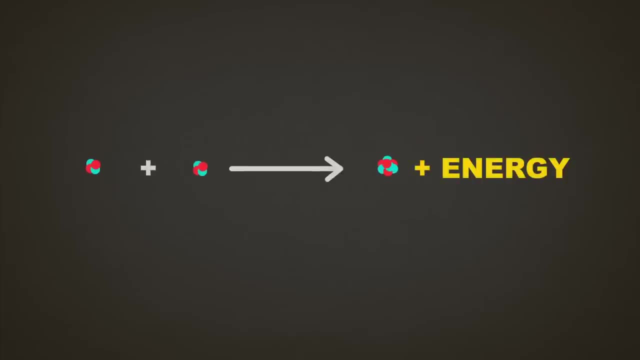 because they release an astounding amount of energy, seemingly out of nowhere. However, thanks to Einstein's famous equation, we know that energy is equivalent to mass. It turns out that the total mass of the starting atoms is very slightly more than the mass of the products. 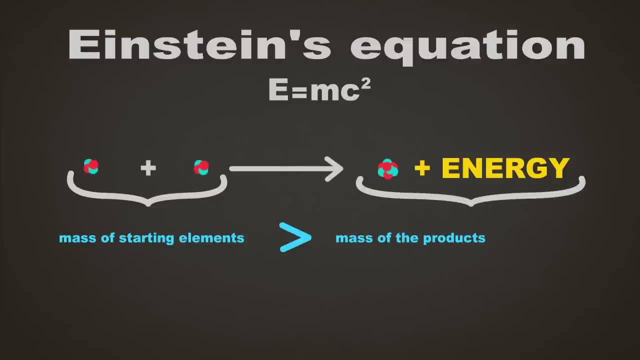 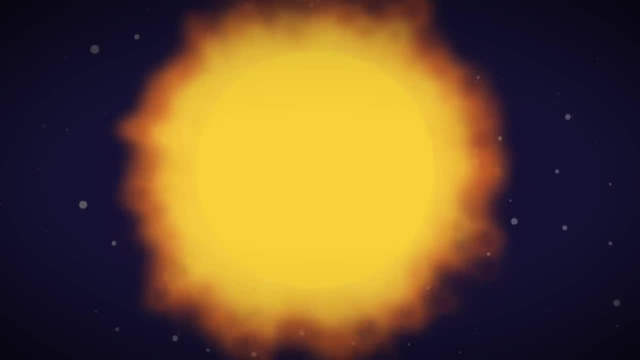 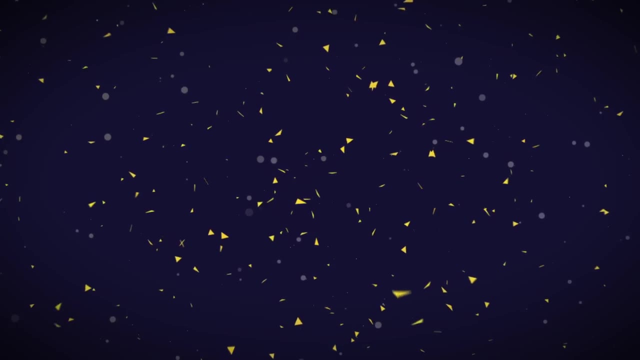 and that loss of mass perfectly corresponds to the gain in energy which radiates out from the star as light, heat and energetic particles. Eventually, this star went supernova and scattered its elements across space. Long story short, they found each other and atoms from other supernovas.